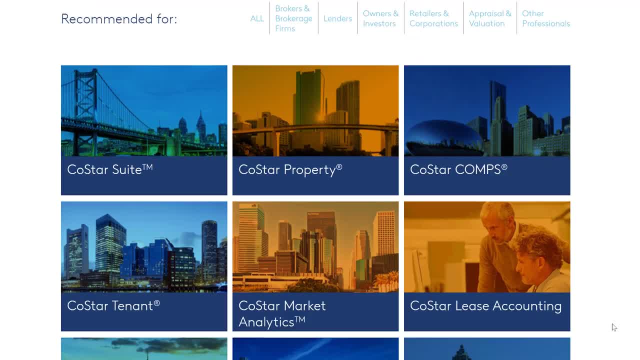 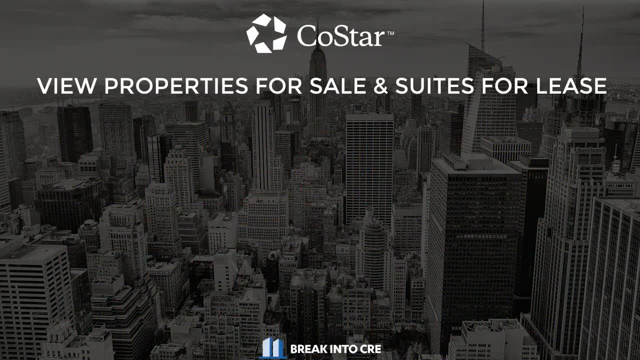 and sale comps for office, retail and industrial properties by both brokerage firms and principal side investors as well. They'll also be able to view properties for sale and suites for lease, including details on property size, year built, upcoming lease expirations. 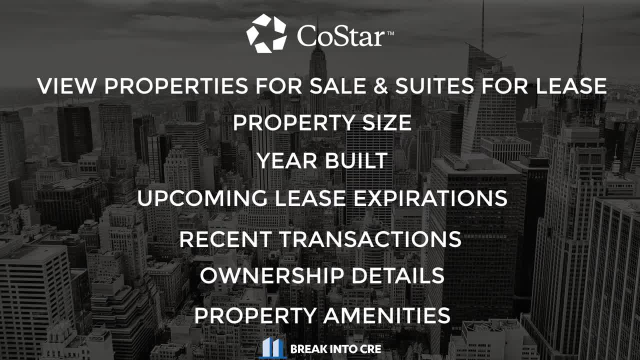 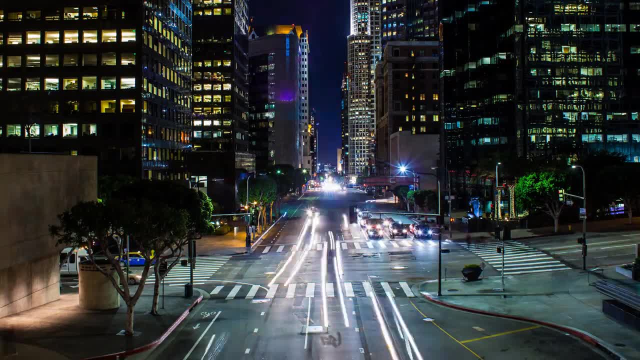 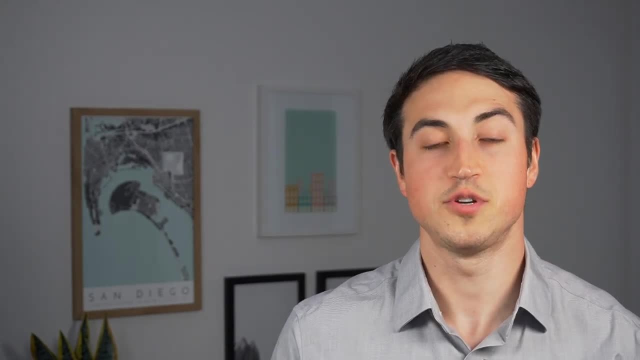 recent transactions, ownership details and property amenities, as well Demographic data and traffic counts are also included in CoStar data, which can be especially helpful when you're analyzing a retail property and want to make sure that the property has an appropriate tenant mix and the traffic count is there. CoStar also allows you to view historical data and forecast for. 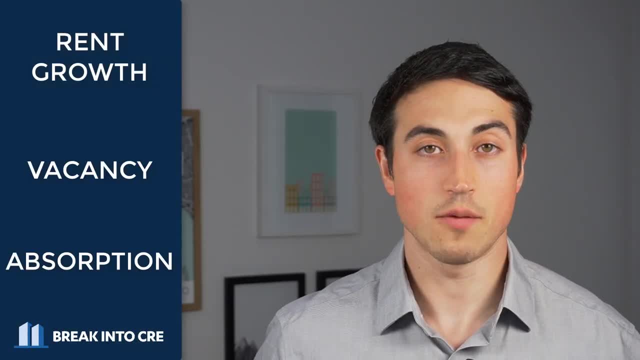 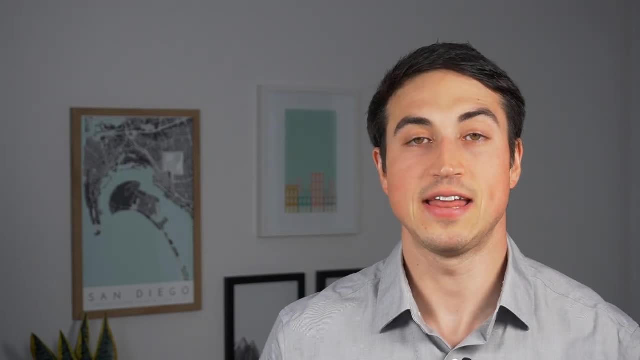 things like rent, growth, vacancy rates and absorption, which is going to help you make your decisions in your real estate financial model that you're projecting 5,, 7 or 10 years out. Now, for retail, office and industrial properties, CoStar tends to be the industry standard, But for 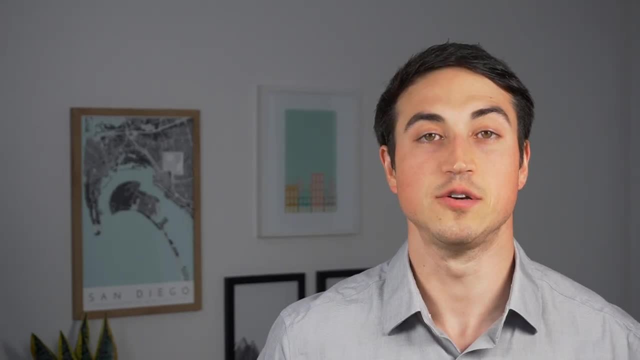 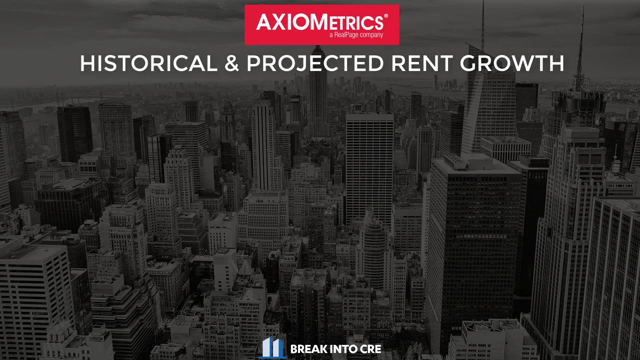 multifamily. there are a few other industry databases that are widely used across the industry, And the first resource is Axiometrics, which is often used to find historical rent growth data and rent growth projections, concessions in the market, job growth, residential permitting for both single family and multifamily units and income levels as well. 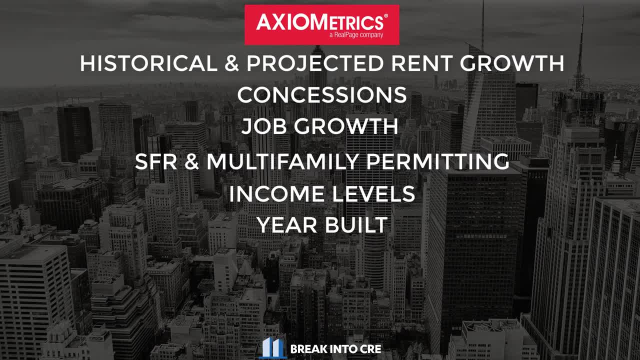 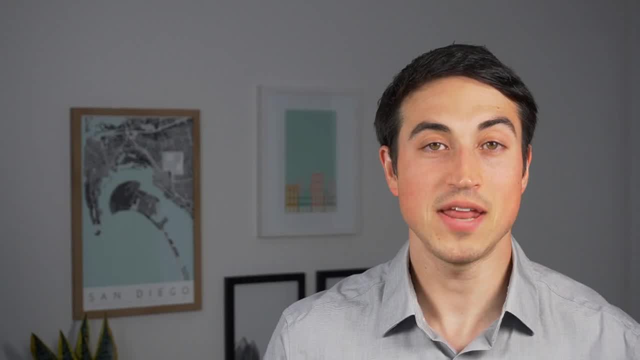 Axiometrics also covers basic property statistics like year built, current rental rates, property class, ownership statistics and rent comps as well. Now, in addition to Axiometrics, many multifamily investors will also use another resource very similar to this, and that is Yardi. 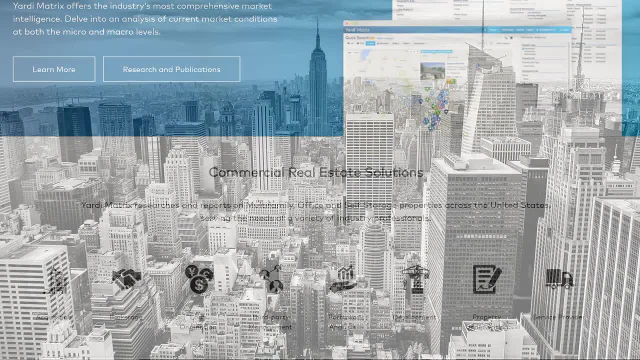 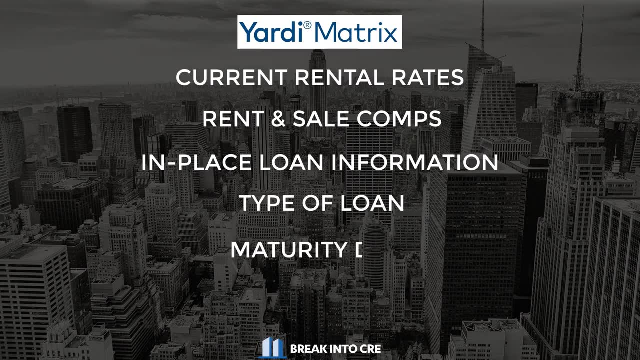 Matrix And Yardi. Matrix includes similar information on current rental rates, rent comps and sale comps, and also includes in-place loan information, including the type of loan, the expiration date and also the rent and occupancy history of each of the properties. So if you're. 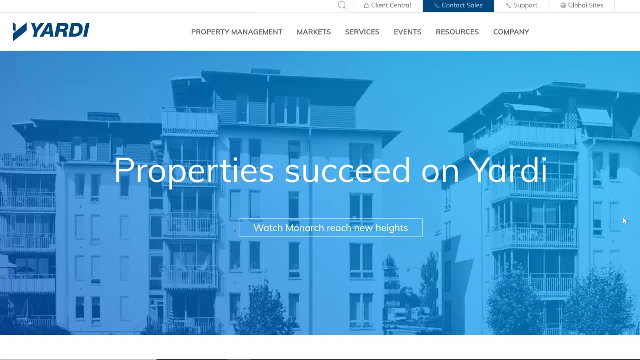 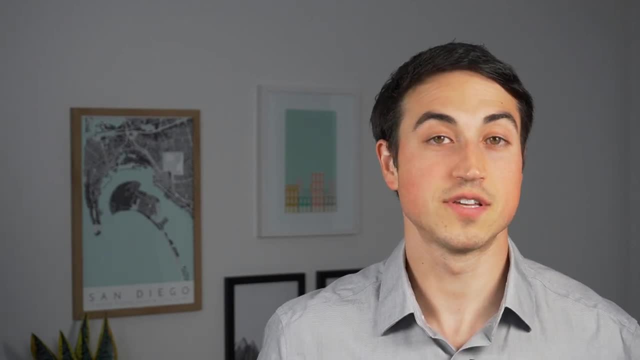 interested in learning more about Yardi, you can go to Axiometricscom and click the link in the description. Yardi is also one of the largest property management software companies in the US, And with that they've been able to aggregate a lot of expense data across thousands of different 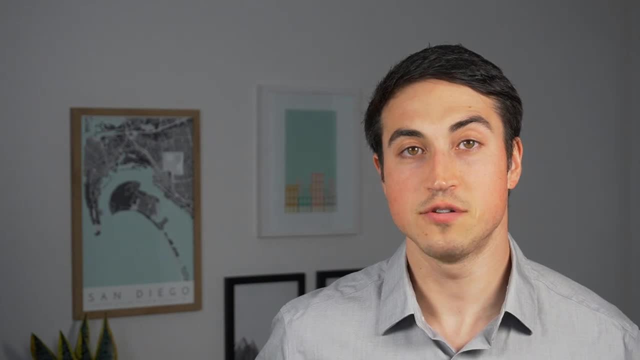 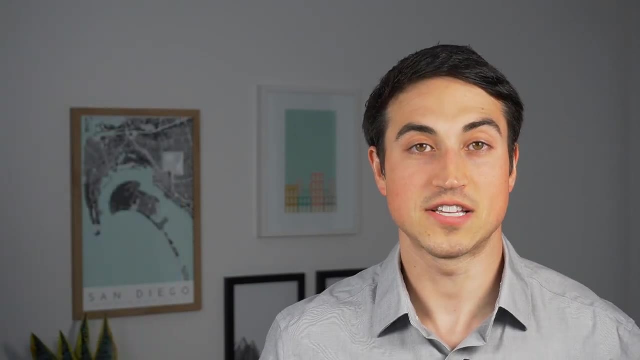 properties in many different markets And because of that, Yardi users are able to see the expense comps of comparable properties in that immediate area, So they can get an idea of the expense loads on a line item by line item basis for comparable properties in the market. Now, finally, for